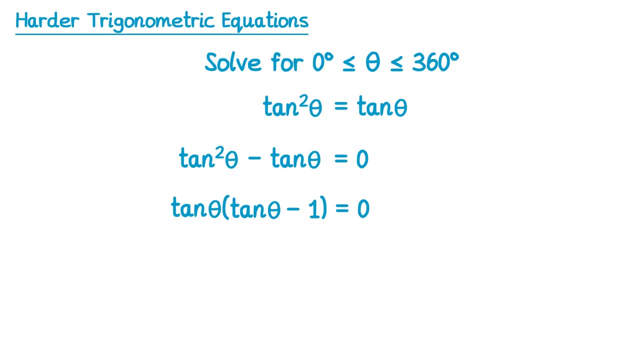 Now here we have two things that are multiplied together that give you 0. So at least one of them must be 0. So we can write two equations from this. Firstly, tan theta here, that could be 0, so tan theta equals 0, or the bracket could be 0, so tan theta minus 1 here, that could be 0. 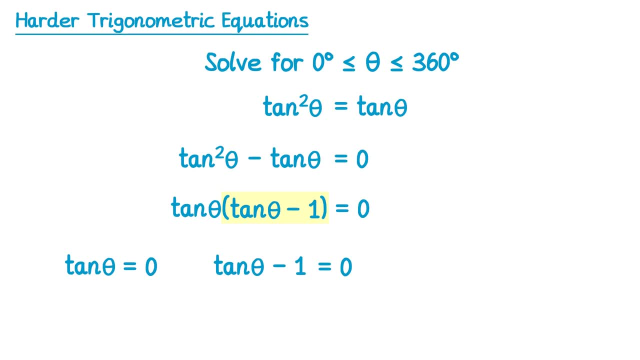 The second of these equations can be rearranged a little bit. If we add 1 to both sides we end up with tan theta. 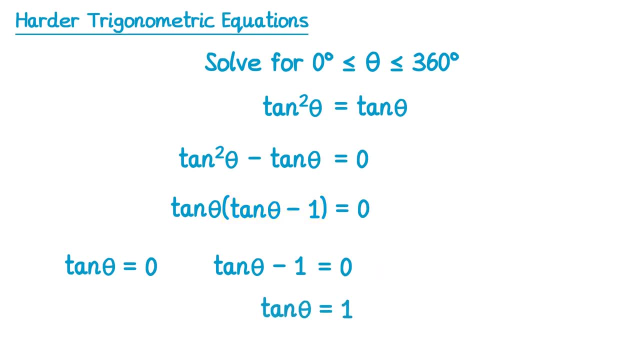 So we've managed to turn this complicated equation into two relatively straightforward equations that you should already be able to solve. We've got tan theta equals 0 and tan theta equals 1. 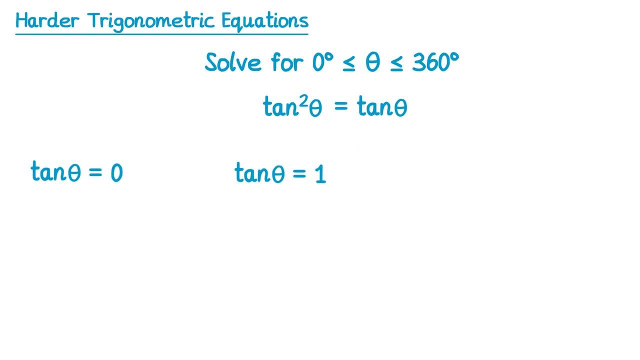 Let's just solve both of those in the usual way. First of all we'll do inverse tan of 0, which is 0, and for the second equation we'll do inverse tan of 1, which is 45 degrees. 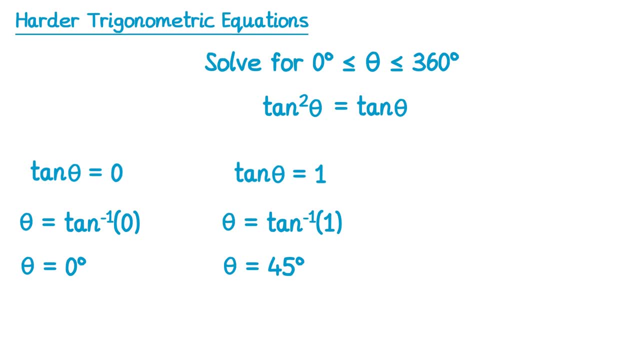 Now we need to use the graph to find the remaining solutions. So let's draw the graph of y equals tan theta. It would look like this. And we'll start with the one where it equals 0. So we draw a horizontal line at 0, and you can see there are three solutions here. One that we already have, which is 0, but also 180 and 360. So we write those solutions down as well. Now what about when tan theta was equal to 1, where we draw a horizontal line at 1? And we can see there are two solutions this time. One of those we already have, that's this one here, 45 degrees. And to get the second one, for tangraphs we add 1 to that. So we'll hand graphs we add 180, so 45 plus 180 is going to give you 225 degrees. So the other solution here is 225 degrees. So all together for this equation there are actually five solutions, three from the left equation and two from the right equation. We would usually write all of these out in ascending order, so theta could be any of these numbers 0, 45, 180, 225 or 360 degrees. 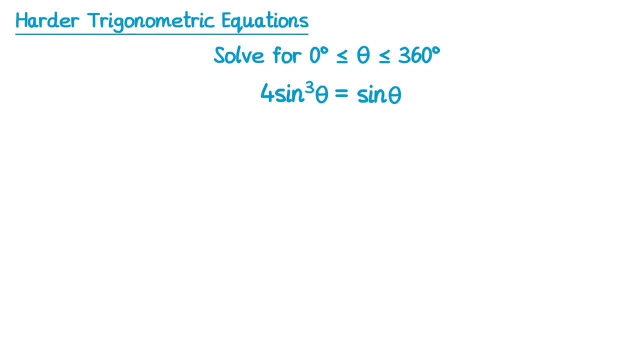 For this equation we're going to use the exact same strategy, so we're going to get all terms on the left hand side and then factorise. So to do this we need to subtract sine theta from both sides. If we subtract it from the left we get 4 sine cubed theta minus sine theta, and if we subtract it from the right the right hand side will just be zero. This time we're going to factorise out all the terms on the left hand side and then factorise. This time we're going to factorise our sine theta, so we get sine theta with a bracket and it's going to equal 0, we just need to work out what goes in the bracket. To get 4 sine cubed theta we need to multiply sine theta by 4 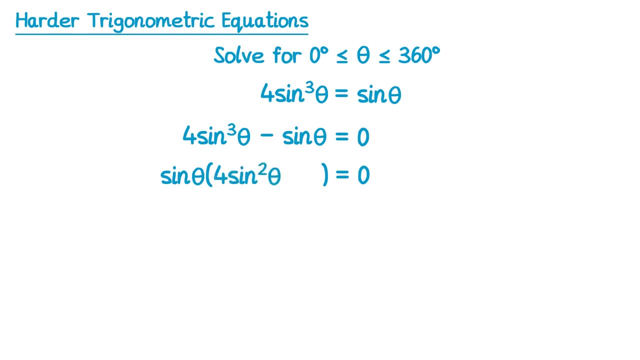 and by sine squared theta, and to get the negative sine theta we just multiply by a negative 1. 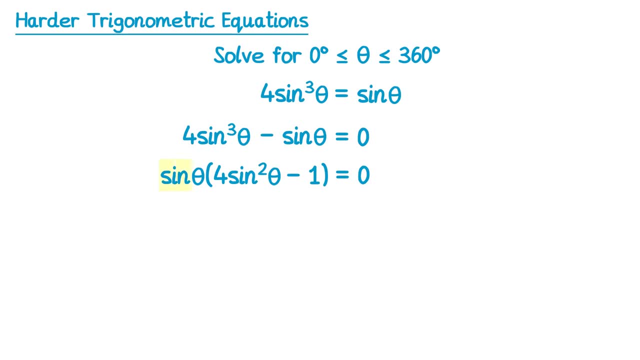 Now we have it factorised again we can see that either sine theta here must be equal to 0, or the whole bracket here must be equal to 0, so 4 sine squared theta minus 1 equals 0. We can rearrange the second one a little bit if we add 1 to both sides we get 4 sine squared theta equals 1, and then if we divide both sides by 4 we get sine squared theta on the left equals one quarter, and finally if we square root both sides, square rooting the left hand side will just give you sine theta, and square rooting the right hand side will give you two values, plus or minus one half. So for this one we actually end up with three equations we need to solve. 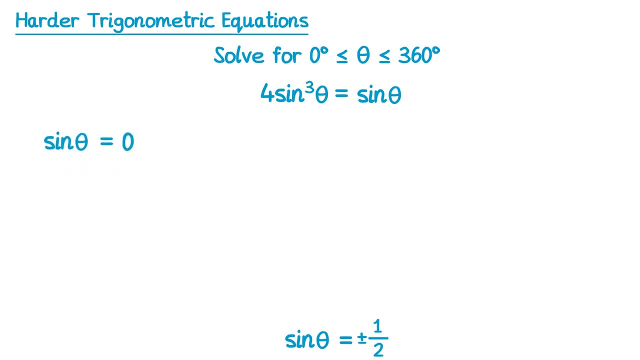 We've got sine theta equals zero, but also sine theta equals zero, but also sine theta equals zero. sine theta equals a half, and sine theta equals negative a half. 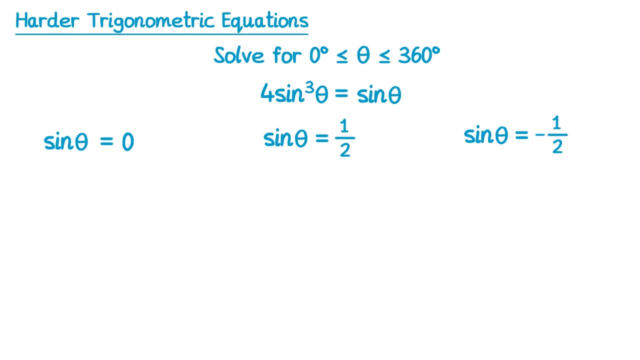 So we're going to solve all of these to get the solutions. We'll start by doing inverse sine of zero, which is zero, and then we'll do inverse sine of one half, which is 30 degrees, and inverse sine of negative a half, which is negative 30 degrees. 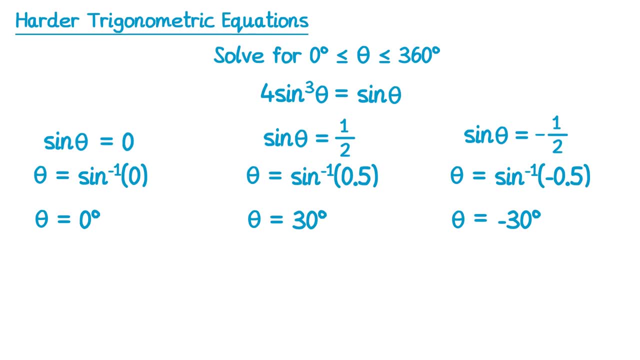 And now we look at the graph to find the remaining solutions. So let's look at the graph of y equals sine theta which looks like this, and we'll start with sine theta equals zero, so if we draw a horizontal line at zero, here you can see there are three solutions. 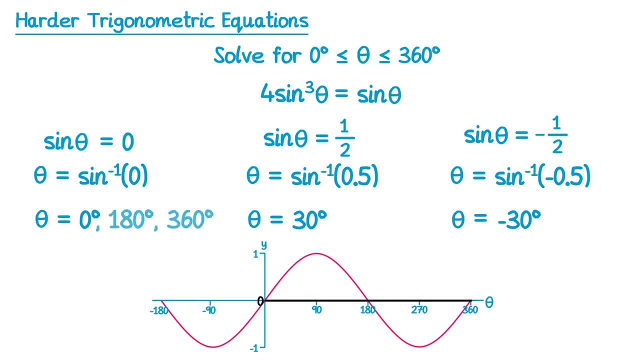 We've already got the one at zero, but we also need 180 again and 360 again. Now let's move on to sine theta equals one half, so we draw a horizontal line at one half, and there are two solutions this time. We already have one of those, that's this one here, 30 degrees, and we need the other one. 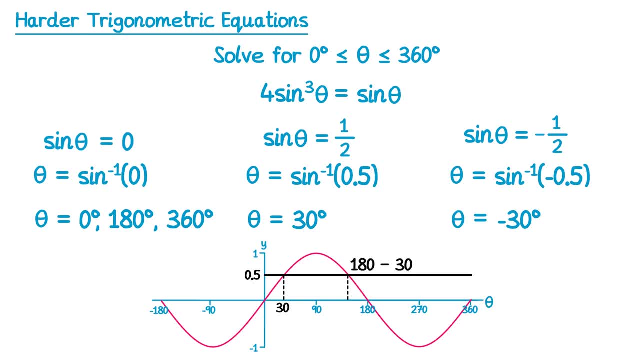 We use the symmetry of the graph to do 180 take away 30, which is 150, so the other solution is 150 degrees. 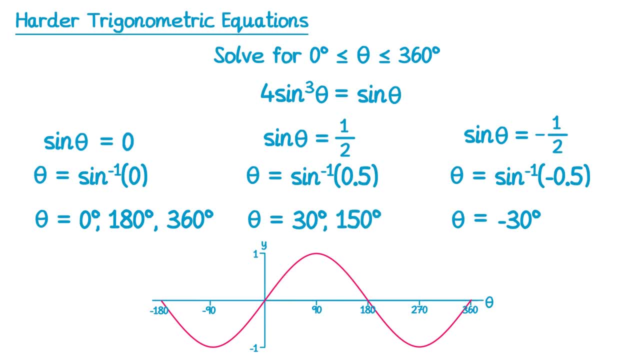 And now we move on to sine theta equals negative one half, so if we draw a line at negative one half down here, you can see the two solutions we want on the right. 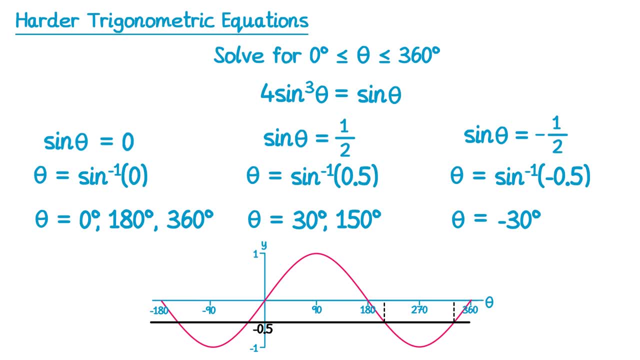 Unfortunately we don't have those, we have negative 30, which is this one here. Now if we use the symmetry of the graph we can find the other solution on the far left here is negative 150, and if we add 360 to both of these solutions we'll get the two solutions on the right. So let's add 360 to both of these, and you'll end up at 210 degrees and 330 degrees. 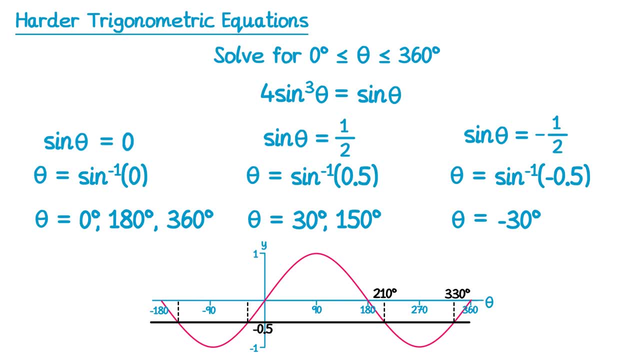 So let's replace that negative 30 since it's outside of the range that we want, with 210 degrees and 330 degrees. So all together for this one we actually have seven solutions. We have 0 degrees, 30 degrees, 150, 180, 210, 330 and 360 degrees. 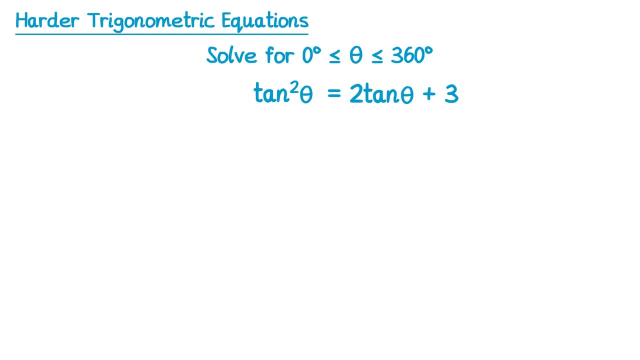 This next question's a little bit harder again. We're going to use the same tactic, we're going to get all terms on the left hand side and factorise. 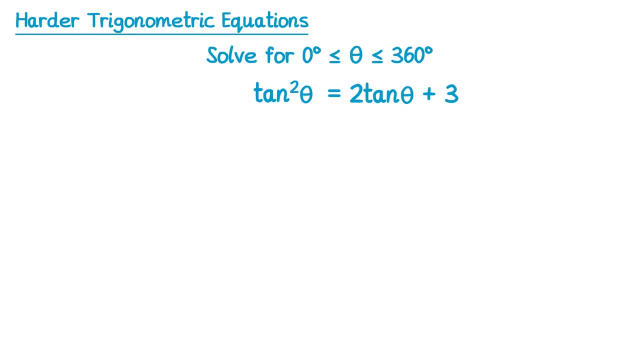 So on the right we have 2 tan theta plus 3, so we're going to subtract that from both sides. If we subtract it from the left hand side, we're going to get 2 tan theta plus 3, so we're going to subtract that from both sides. 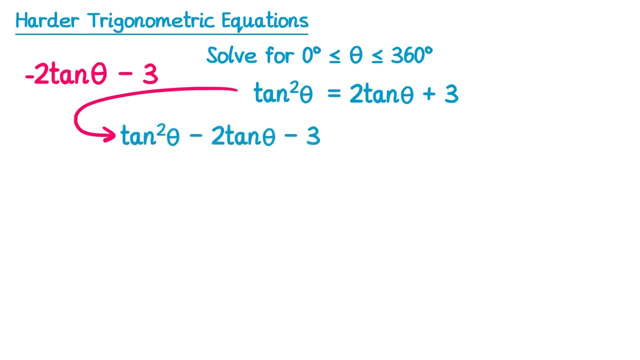 If we subtract it from the left, we get tan squared theta minus 2 tan theta minus 3, and if we subtract it from the right, you guessed it, we get 0. 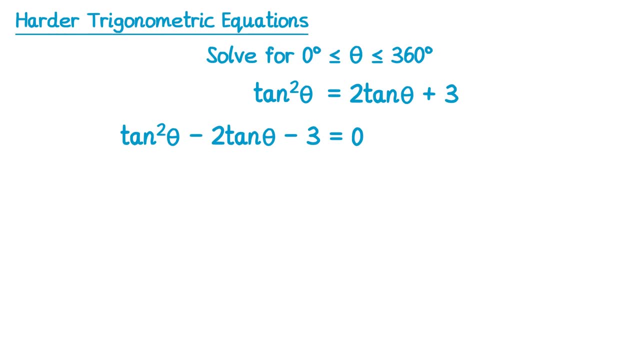 Now we're going to factorise this left hand side, but this one's a little bit harder. It looks a little bit like we've got a quadratic here, and in fact we do, it's just in disguise. So what we're going to do is use a substitution. We're going to imagine that x equals tan theta, in which case tan squared theta is just the same as x squared, and negative 2 tan theta is the same as negative 2x, and then we have negative 3 equals zero. 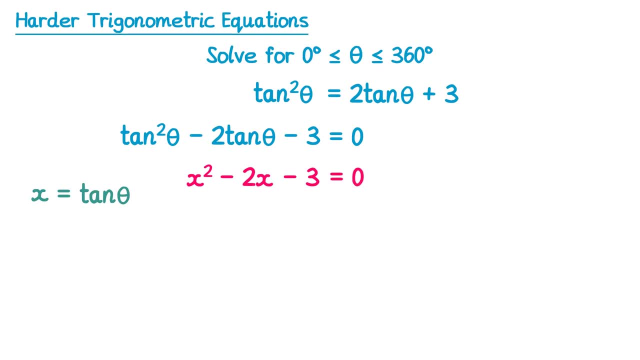 So we've changed this question into a usual quadratic that you will be more comfortable with. 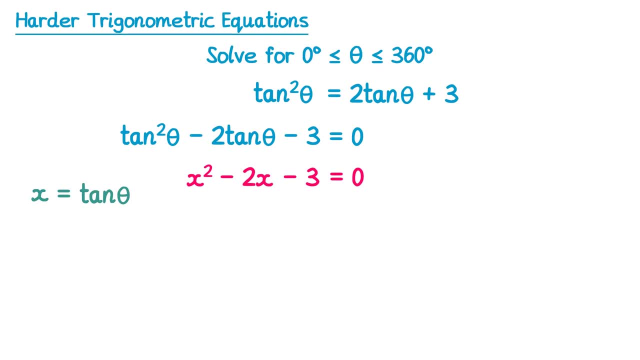 This one factorises quite nicely, it's x take 3 x plus 1 equal 0. Now, if this one factorises, the trigonometric one must also factorise in the same way. Remember we wrote down that x was equal to tan theta. So we can replace the x in the brackets that are factorised with tan thetas. So instead of x take away 3, it's tan theta take away 3, and instead of x take away 3, it's tan theta take away 3. esus is divided by the square root of x squared, constant atualised by x squared, is negative x squared, which equals negative 2 tan theta, so negative 2 and having everything 최 instead of x plus 1 is tan theta plus 1, and this equals 0. You may prefer to write this down each time but eventually you will become more comfortable with factorising these straight away. 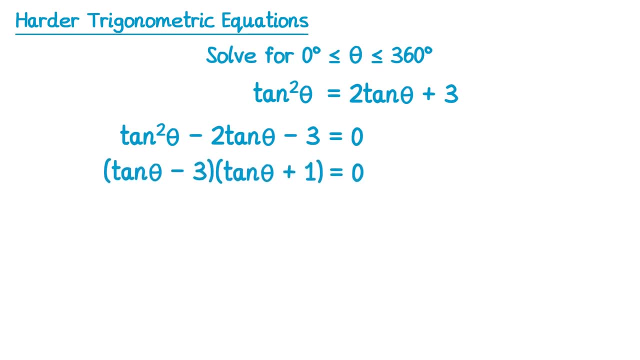 So now that we have it factorised, we can see there are two parts to this solution, we either have the first bracket equal to 0, so tan theta minus 3 equals 0, or the second part, so tan theta plus 1 equals 0. We can rearrange both of these, for the left one we'll add 3 to both sides, this will give us tan theta equals 3, and for the right one we subtract 1 from both sides, so tan theta equals negative 1. We can find some solutions by doing inverse tan, so if we do inverse tan of 3 we end up with 71.6 degrees and inverse tan of negative 1 gives you negative 45 degrees, which isn't in our range unfortunately. Now I'm not going to draw the graph this time, you should already be comfortable now with finding the remaining solutions. For tan graphs we just add 180, so if we do 71.6 plus 180, we'll get the other solution here, 251.6, and for the right equation, negative 45 plus 180, that gives you 135, which is in our range, and you can add 180 to that again, so 135 add 180 gives you 315. Those are all of your solutions, and that equation is now solved. 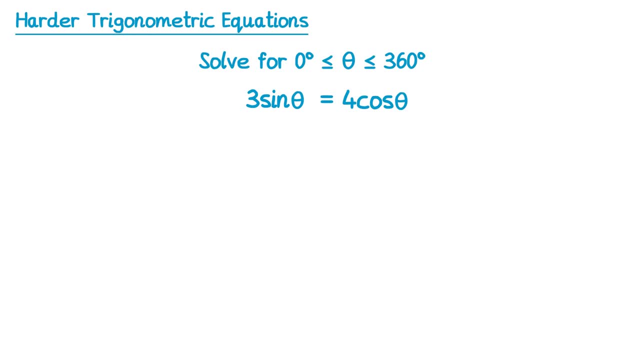 Sometimes we need to use identities to help us solve equations. For this equation here I'm going to start by dividing both sides by cos theta, on the left I'll have 3 sin theta divided by cos theta, and on the right the cos theta's will cancel leaving me with just 4. I'm then going to divide both sides by 3, so on the left the 3 will cancel so sin theta over cos theta, and on the right it will be 4 over 3. Now why have I done this? Well sin theta over cos theta is equal to tan theta, that's an identity that you would have seen in the identities video, so we can replace that with tan theta. Now we have a really straightforward equation to solve. We do inverse tan of 4 over 3, which gives you 53.1 degrees, and to get the second solution since it's tan again we just add 180, so you get 233.1 degrees, and that's that equation solved. 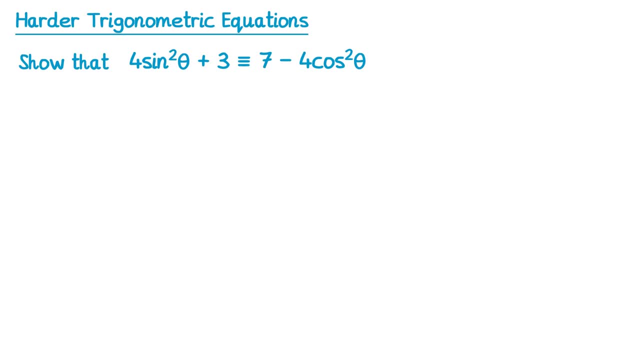 Now sometimes the identities are not so straightforward, so take this question, we haven't actually been asked to solve anything yet, we've just been asked to show that this is true. So we'll start with the left hand side of the identity, 4 sin squared theta plus 3, and we're going to try and end up with the right hand side. What I'm going to do is change the sin squared theta into 1 minus cos squared theta, so I've got 4 lots of 1 minus cos squared theta plus 3. If I expand this bracket, 4 times 1 is 4, and 4 times negative cos squared theta is negative 4 cos squared theta, and then plus 3. You can then collect up the 4 and the 3 to make 7, so it's 7 minus 4 cos squared theta, which is what we needed to show. 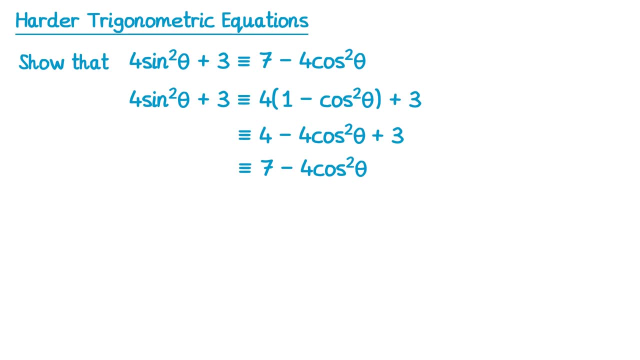 Now sometimes you'll have this as a part a to a question, and then you'll have a follow-up part b that looks something like this. You'll have this as a part a to a question, and then you'll have a follow-up part b that looks something like this. 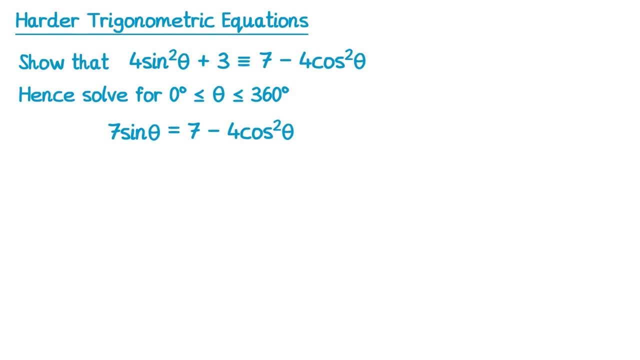 Hence solve this equation. Now if you look carefully at the equation we've been asked to solve, and then you compare that to the identity, you'll see the right hand sides are the same. 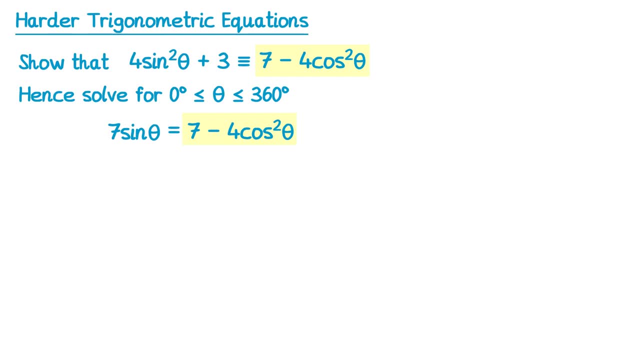 This means we can replace the right hand side of our equation with the left hand side of the identity up here. So instead of writing 7 minus 4 cos squared theta, I'm going to write 4 sin squared 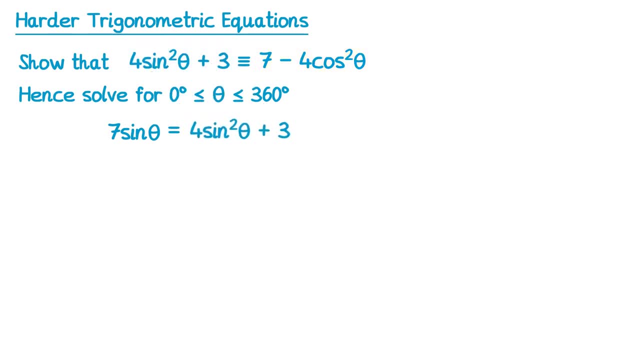 theta plus 3, like this. The advantage here is that we've now got an equation that only has sines in it. So I'm going to get all of the terms on the same side, this time I'm going to go for the right hand side, 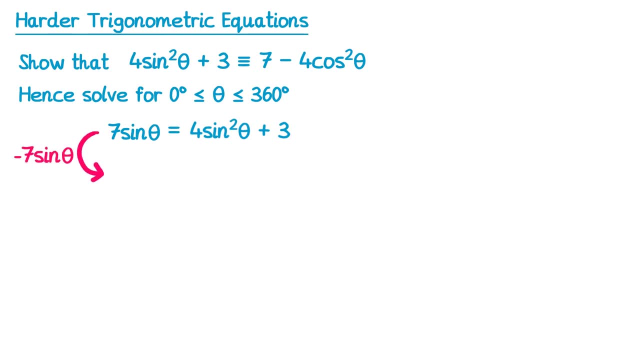 so I'll subtract 7 sin theta from both sides. If I subtract it from the left I get 0, and if I subtract it from the right we get 4 sin squared theta minus 7 sin theta plus 3. This is another quadratic that we can factorise. 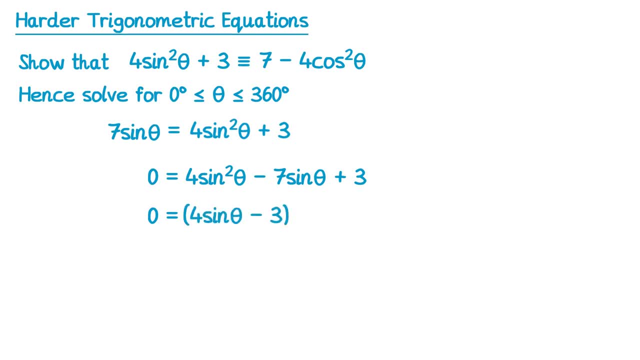 So if we factorise this one we end up with 4 sin theta minus 3, and sin theta minus 1. Now we just set each of the brackets equal to 0, so the first one, 4 sin theta minus 3 equals 0, and the second one, sin theta minus 1 equals 0. 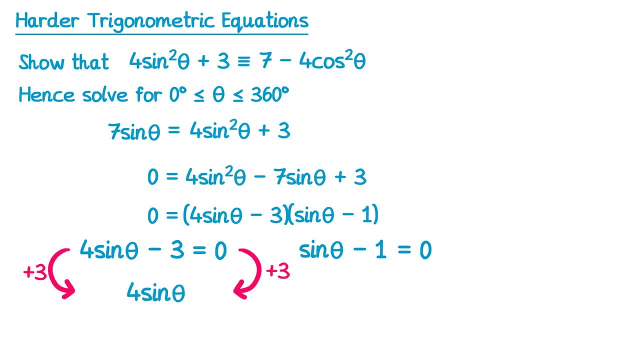 For the left one we add 3 to both sides, that gives you 4 sin theta equals 3, and then divide by 4, so sin theta equals 3 quarters, 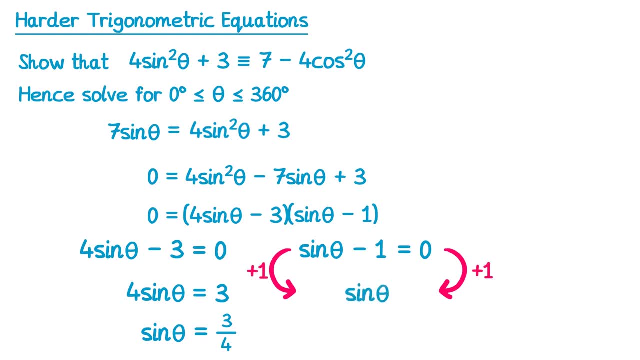 and for the right one we just add 1 to both sides, so sin theta equals 1.